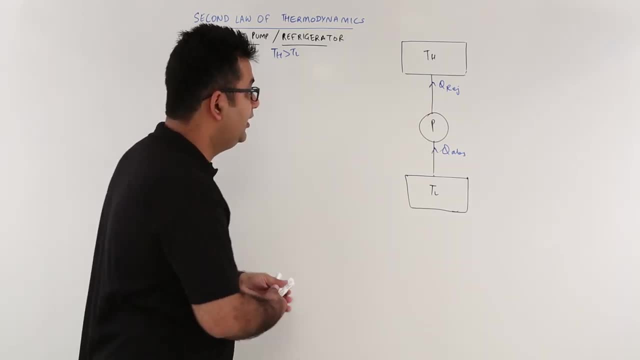 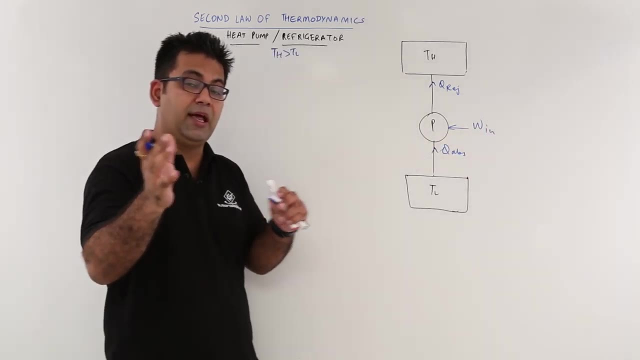 flow of heat without any work input. So to maintain this, you have to have a reverse flow of heat without any work input. To maintain this you need to provide some energy input in form of work. So, if you put it, analogous to the water pump. So to run a water pump you need to provide some electrical. 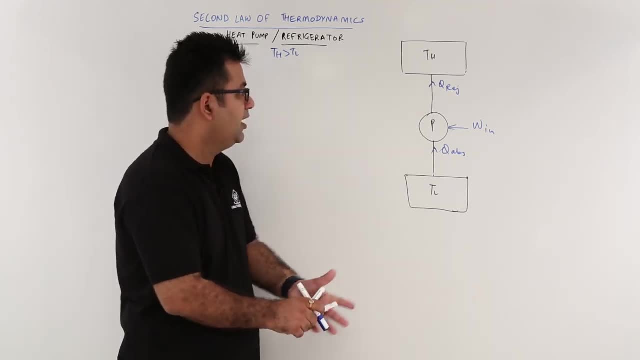 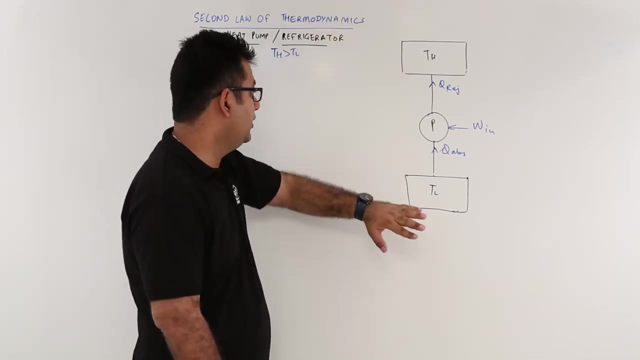 energy. So you have a small motor with it. That motor provides work input, that it picks up water from low level and throws it to a high level. Okay, So the similar thing is happening in heat pump. You put in some work energy. It picks up heat from low temperature. 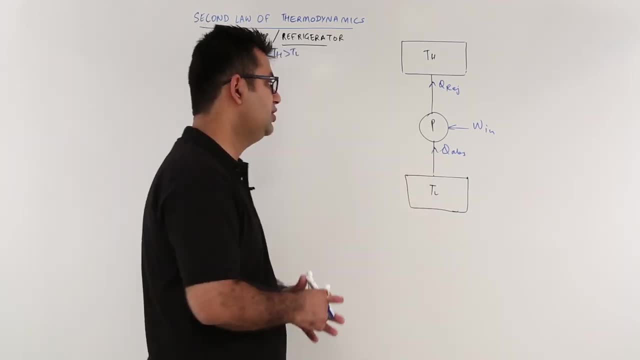 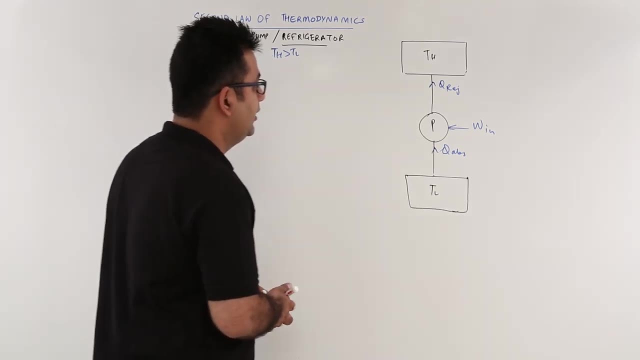 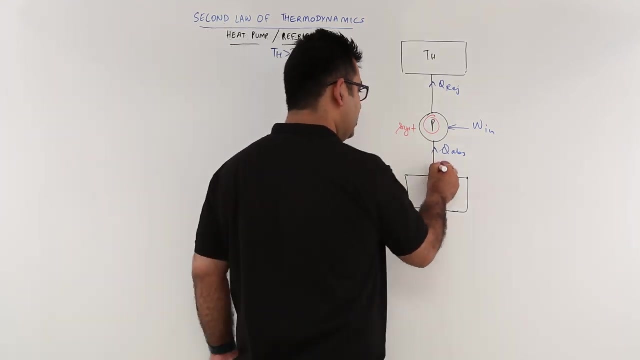 So this is the schematic and the concept of heat pump. Now, if you look at this, the pump is now a system that we want to study. Okay, In the system you have these two energies coming in, So the energy which is coming into the system is absorbed: heat plus work. 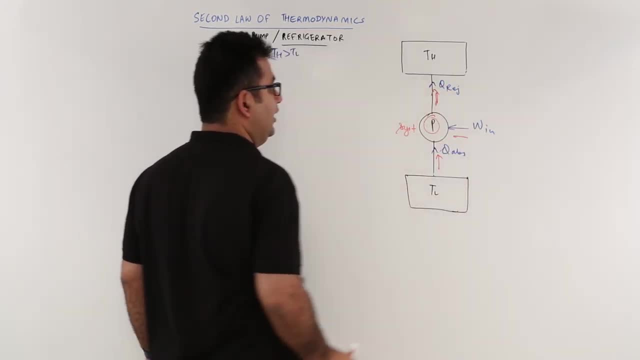 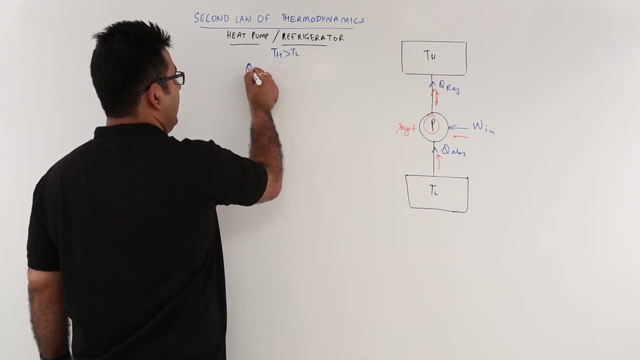 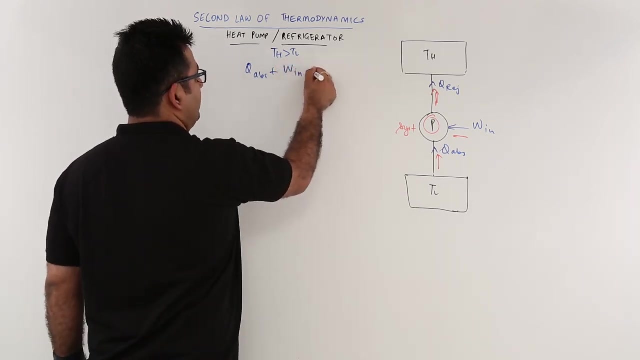 input And what goes out is the heat rejection. Okay, So, yes, that is the system. So you have the heat rejection. Yes, that is quite peculiar because you will have higher heat rejection as compared to heat absorption. Okay, So you have W input. This is equal. 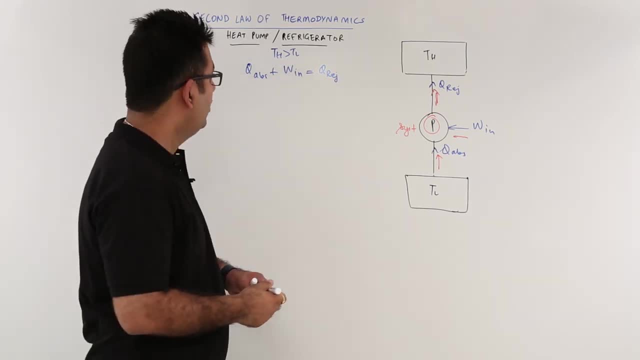 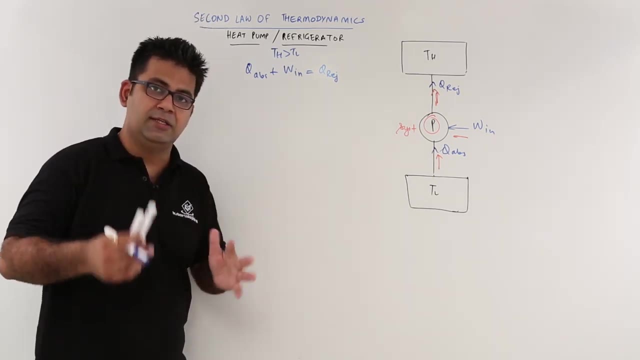 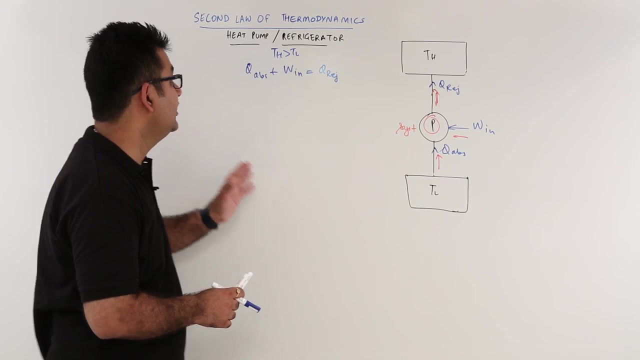 to Q rejected. Okay, So this is the energy balance in the case of a heat pump. Now for a heat engine. you had efficiency to actually understand and gauge the performance of that heat engine. In this case we do not use efficiency because efficiency is somewhat output upon input. 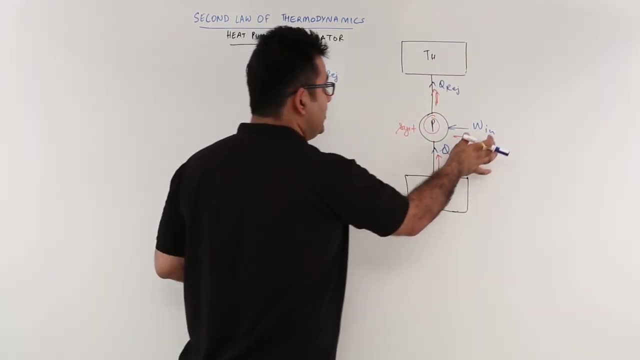 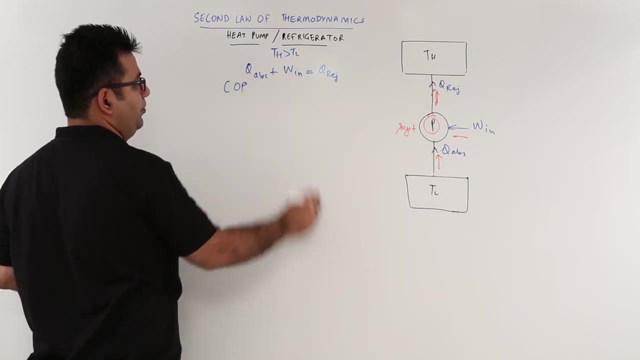 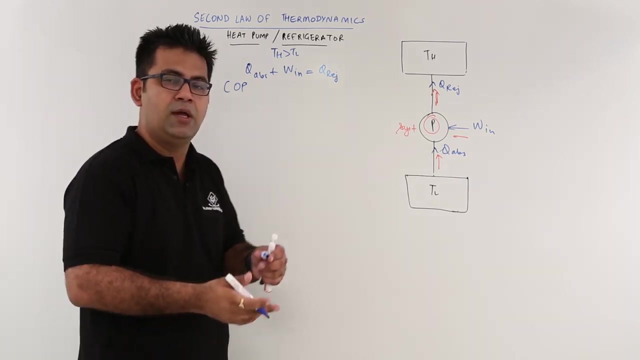 And that output that you had in heat engine is being used as an input in this case. So the whole thing reverses. So in this we use a term, COP. COP means coefficient of performance. This coefficient of performance or COP, it gives you a measure of the performance of. 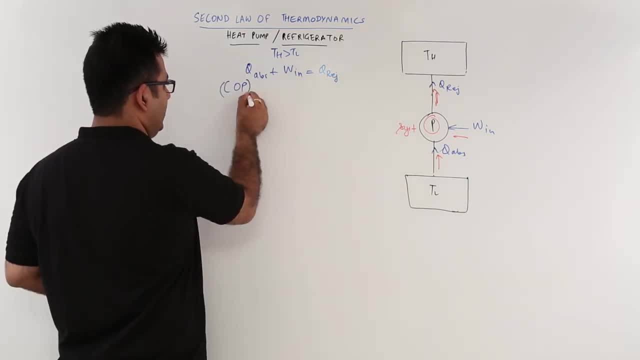 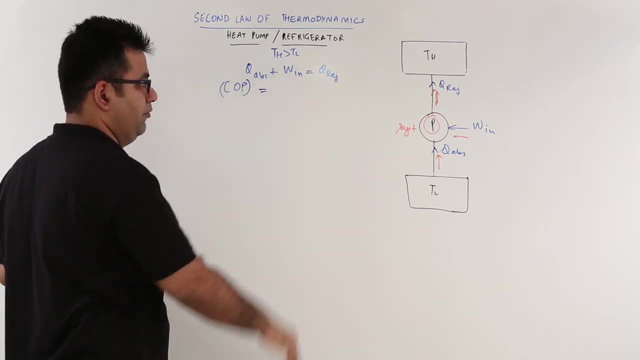 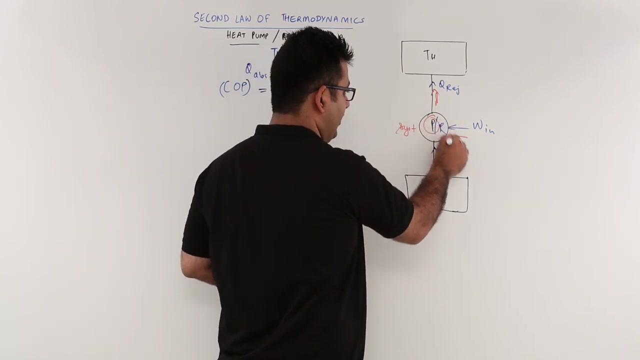 this heat pump. Okay, So let me put P over here, which denotes pump. This is equal to So in general, if you talk about. let me just remove it, because for a refrigerator also, this is the same schematic, but in place of P I will write R. Okay, So you will have a COP for a pump. 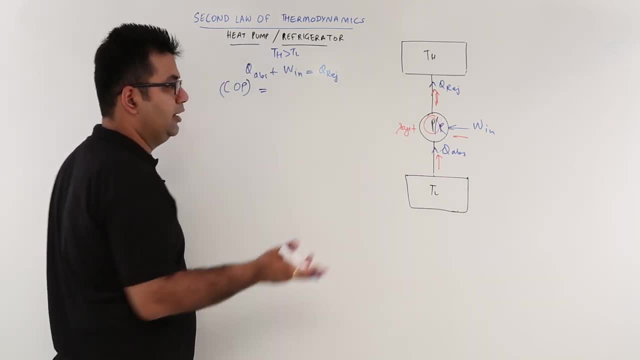 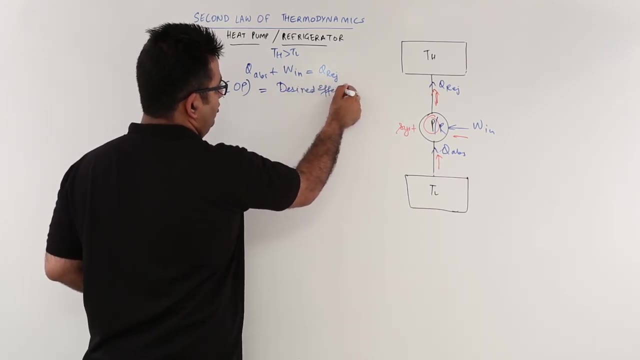 and a COP for the refrigerator. So in general, the COP means it is the ratio of the desired effect you want to have. Okay. So this is the ratio of the desired effect you want to have. Okay. So in general, the COP means it is the ratio of the desired effect you want to have. 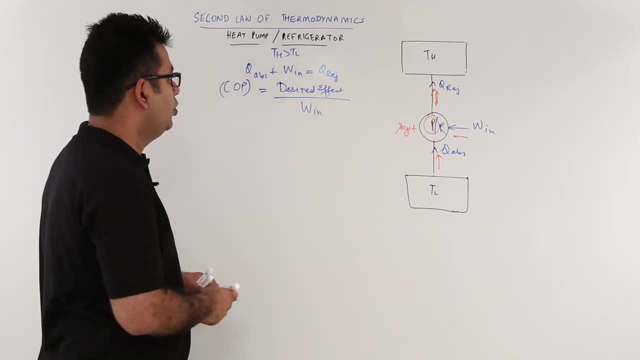 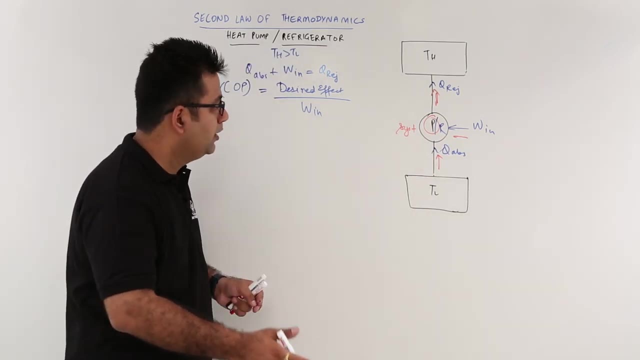 Upon the energy input, that is, spark input. Okay, So what is the desired effect in case of a pump? first of all, Now, with the pump, we want that the. you know, if you put it analogous to the water pump, you want that that water pump should supply water to the. 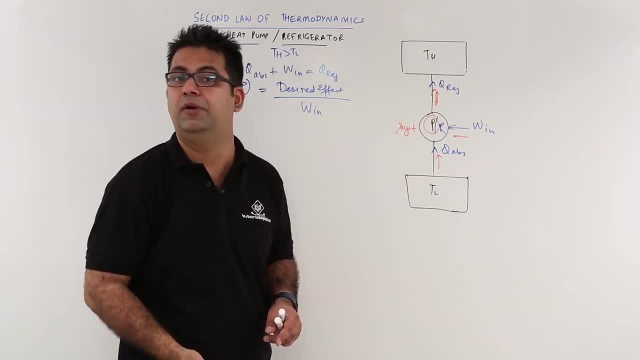 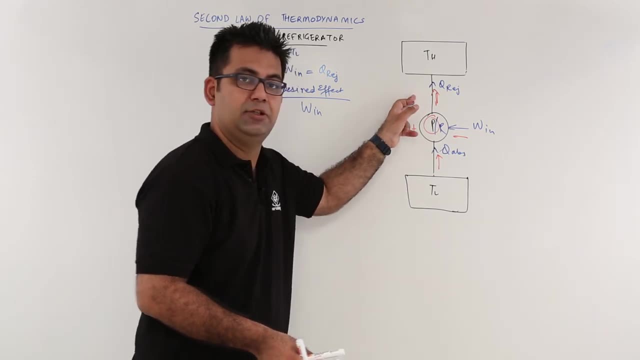 highest possible level with the lowest possible amount of energy input. You want your COP to be as high as possible, So the desired effect becomes heat rejection. So you want as high heat rejection as possible, So you want the desired effect to be as high as possible. 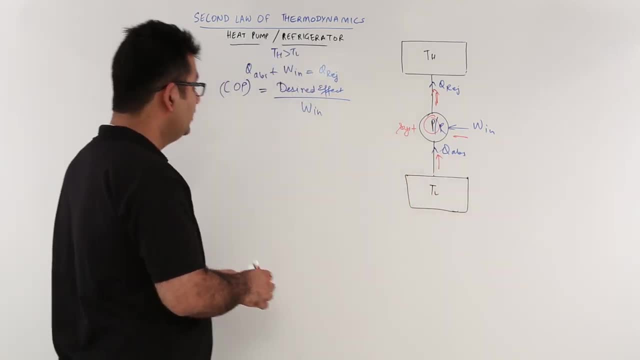 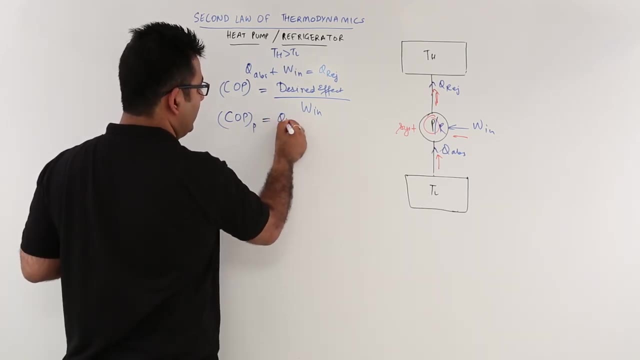 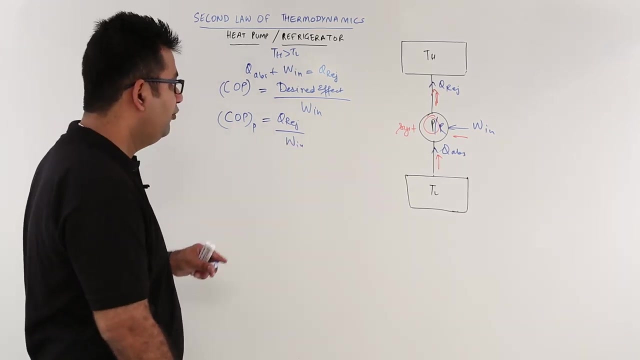 With the lowest amount of work input, Okay. So in this case, that is the case of COP of a pump, the desired effect becomes the heat rejection upon work input. Okay, Now if you talk about refrigeration or refrigerator. refrigerator means you need to absorb as much. 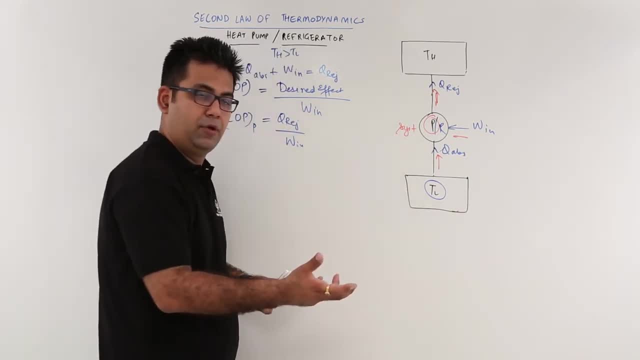 amount of heat as possible from a substance, because you need to cool this place. That is the amount of heat that you need to absorb from a substance, So you need to cool this place. That is the function of this, because this, will you know, be taught in the topic. 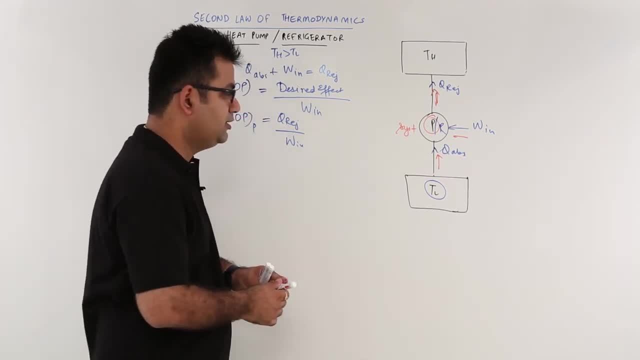 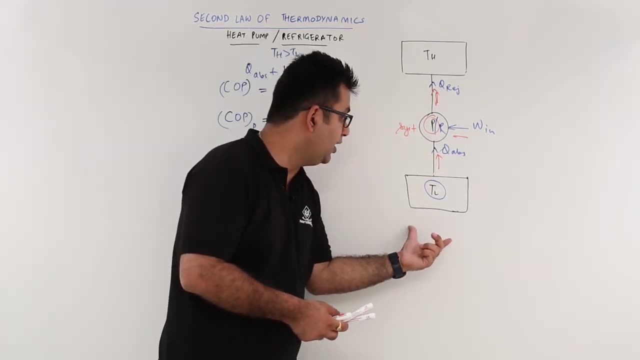 of RAC in detail. That is a separate subject altogether. But just understand this. With the refrigeration, we want to achieve maximum cooling here. How do you achieve cooling here? You achieve cooling here by extracting heat from this particular area. You want maximum. 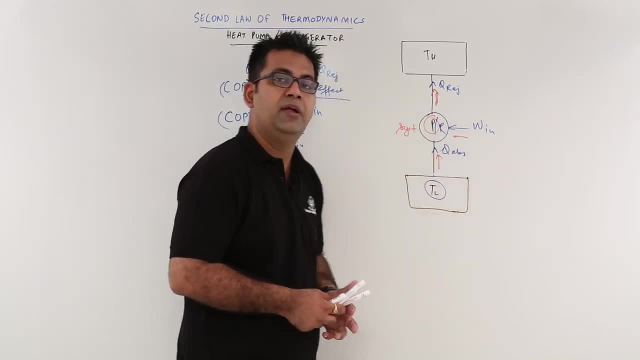 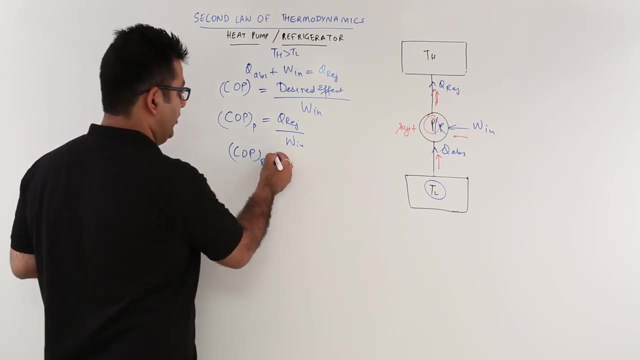 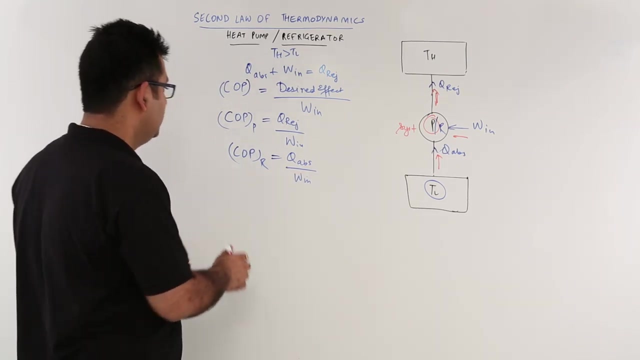 amount of heat absorption by minimum amount of work input. So the COP, you know you want maximum amount of heat absorption by minimum amount of work input. Okay, So this is a concept worth noting and understanding in detail. That is the difference between: 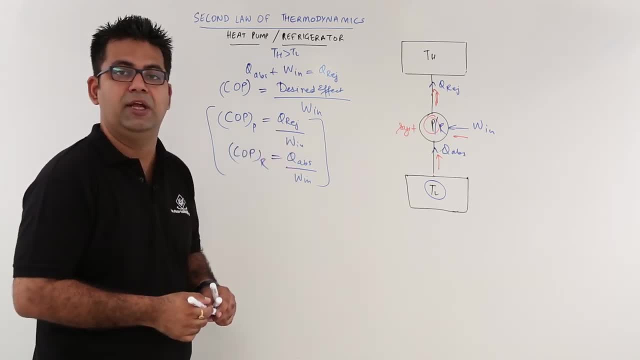 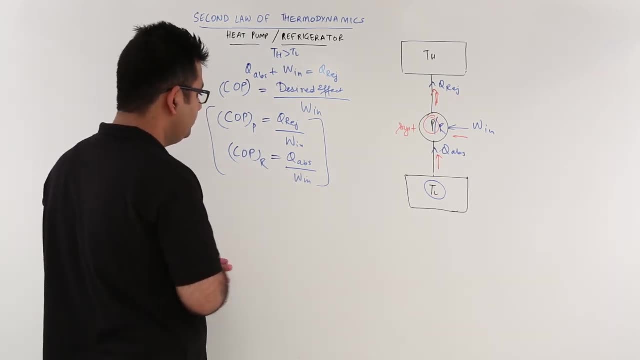 a refrigerator and a heat pump and then comparing it with heat engine. Okay, Now what is the relation? There has to be a relation between these two. Okay, If you look at this equation, let us bring it down. So you have Q.